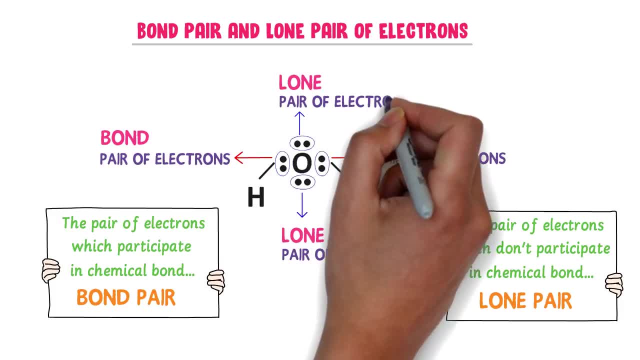 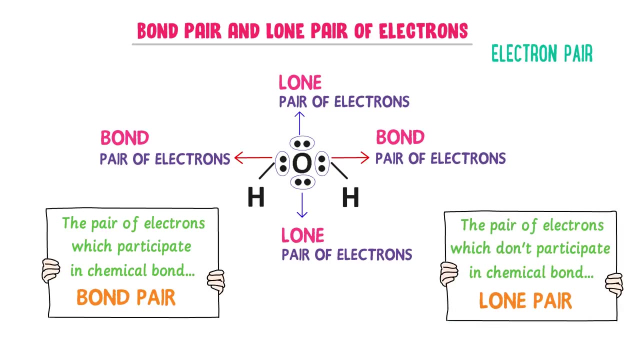 electrons are called lone pair of electrons because they do not participate in chemical bond. Thus water has two bond pair of electrons and two lone pair of electrons. Therefore, whenever I say electron pairs in this lecture, you must remember that either it means bond pair of electrons or lone pair of electrons. Secondly, to learn whisper theory, we must 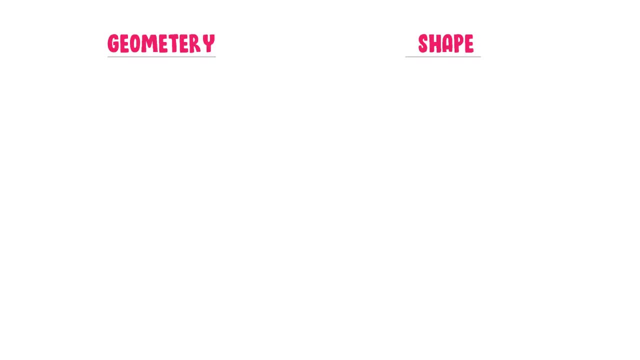 also learn the difference between the geometry and shape of molecules. Remember that the shape of any molecule is determined by the shape of the molecule. So if we have a molecule in the shape of the molecule, then its shape is recorded as shape ofenda. 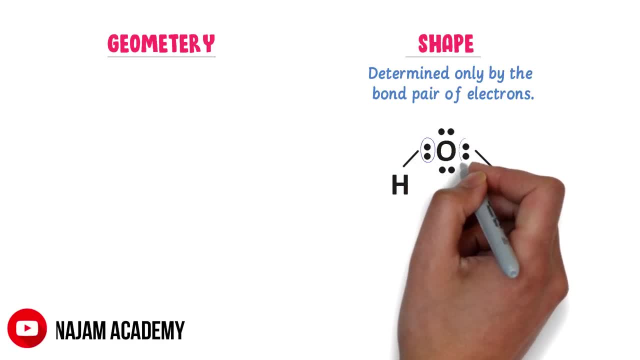 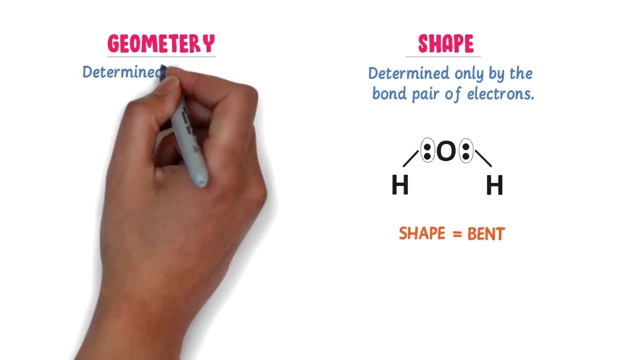 So basically a unique location of the molecule is recorded, to be located in the shape of the molecule. For that we need to work on the bleach outcome for the biochemicals. It is basically Когда se attrub of water. we consider two bond pairs and two lone pair of electrons. 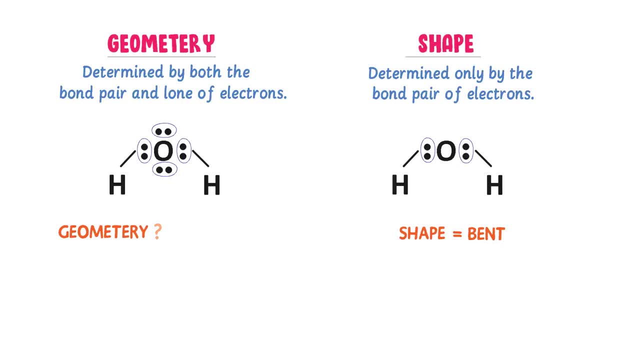 Now can you guess the geometry of a water molecule? Well, it is tetrahedral. Just note it down that shape of a molecule is determined by the bond pair of electrons and geometry of a molecule is determined by both bond pair and lone pair of electrons. 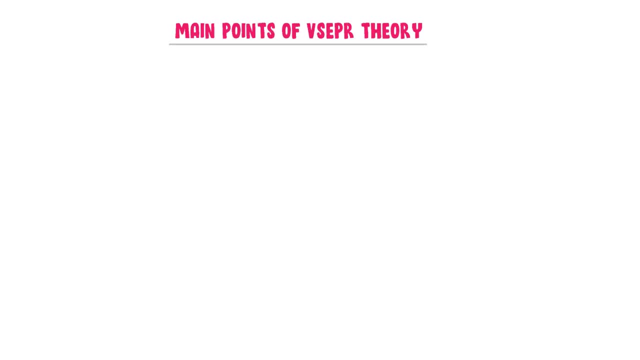 So let me quickly teach you the postulates or main points of Whisper theory. Remember that Whisper stands for Valence Shell Electron Pair Repulsion. The first point of Whisper theory states that electron pairs repel each other and tend to stay away. 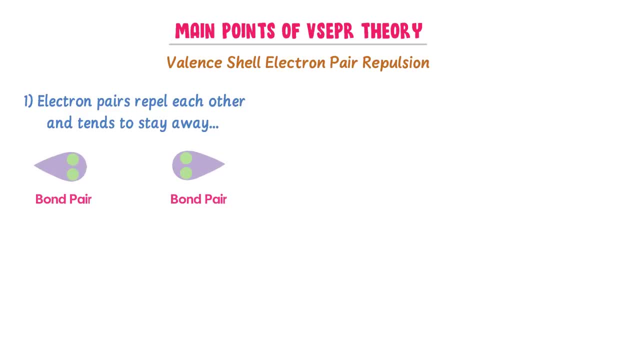 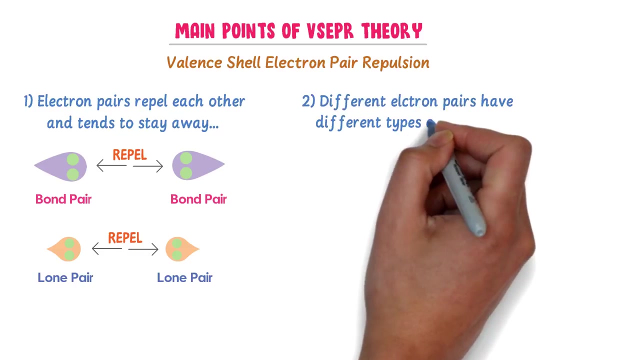 For example, consider this bond pair and this bond pair of electrons. These both pair of electrons repel each other because electrons are negatively charged and, like charges, repel. Similarly there is repulsion between these London pair of electrons. The second point of Whisper theory states that different electron pairs have different 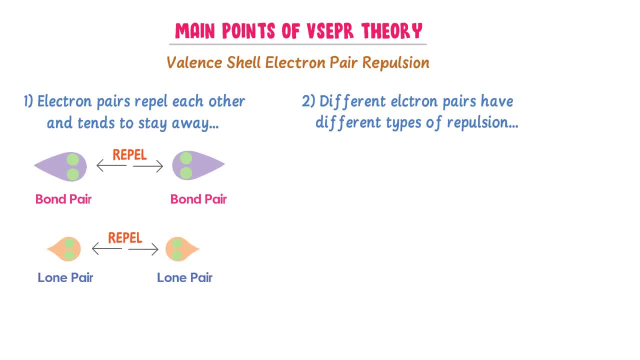 types of repulsion. There is maximum repulsion force between London and London pair of electrons. There is less repulsion force between London pair and bond pair Of Electrons And also very less repulsion force between London and London pair of electrons. 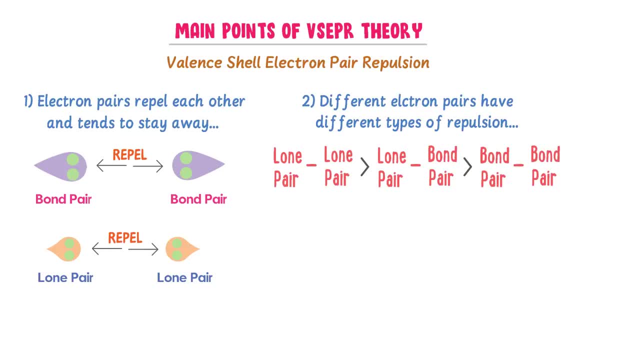 Thanks for watching. bond pair and bond pair of electrons. The third point of Fisper theory states that geometry and shape of a molecule is determined by the bond pair and lone pair of electrons. The fourth point of Fisper theory states that if lone pair is zero in a molecule, 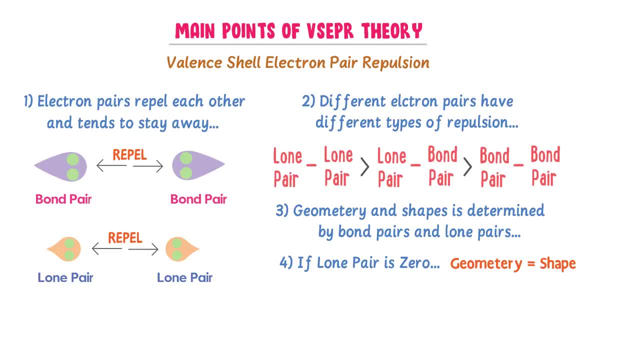 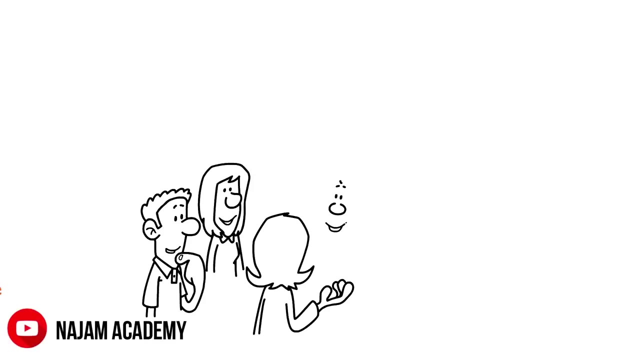 then both the geometry and shape of a molecule is the same. If lone pair is not zero in a molecule, then the geometry and shape of a molecule is different. Thus noted down these main points of Fisper theory. Now in the exam we are usually asked to find bond pair of electrons. 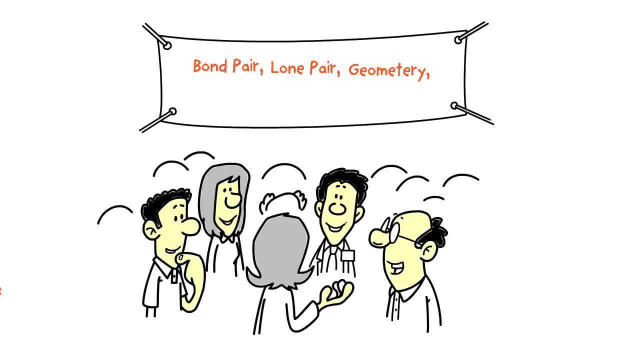 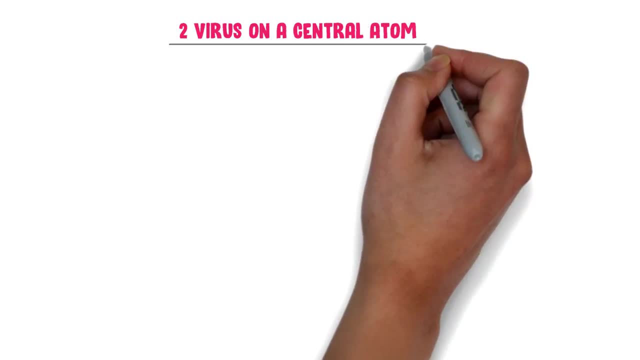 lone pair of electrons, geometry of a molecule, shape of a molecule, hybridization and bond angle of a molecule. Hence I will teach you some important molecules which would help you a lot. Consider molecules which have two atoms on central atom, but personally I say two virus on a central atom. 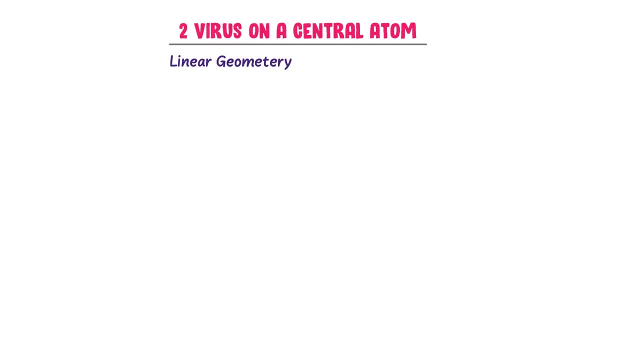 The geometry of these types of molecules is linear and they have sp hybridization. Remember that geometry of these molecules remain the same and never changes, even if the shape changes. For example, consider a molecule like beryllium chloride- BeCl2.. 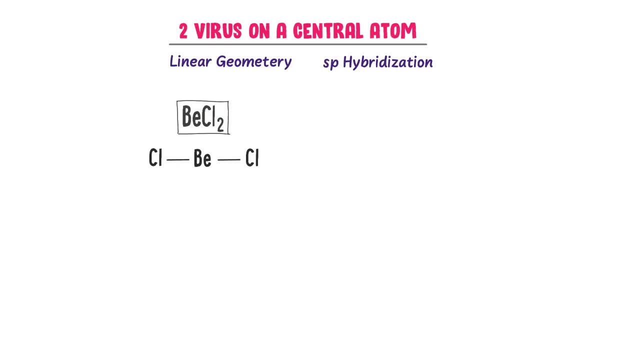 The Lewis structure of this molecule is like this: Beryllium forms 2 single bonds with chlorine, So the bond pair in this molecule is 2.. There is no lone pair of electrons present on central atom, So the lone pair is equal to 0.. 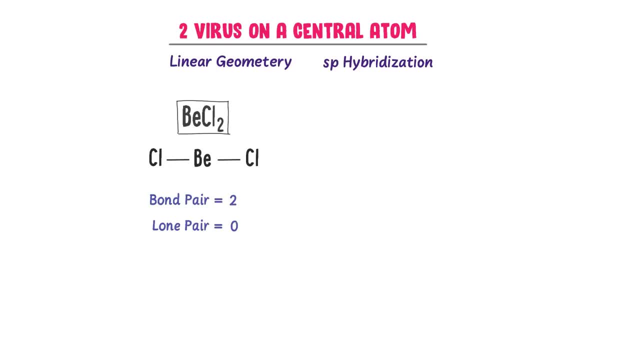 According to Fisper theory, when lone pair is zero, the shape of a molecule is the same as its geometry. Thus the geometry of this molecule is linear. Also, ship is linear. Beryllium forms two bonds, so it contains SP hybridization. The bond angle is 180. 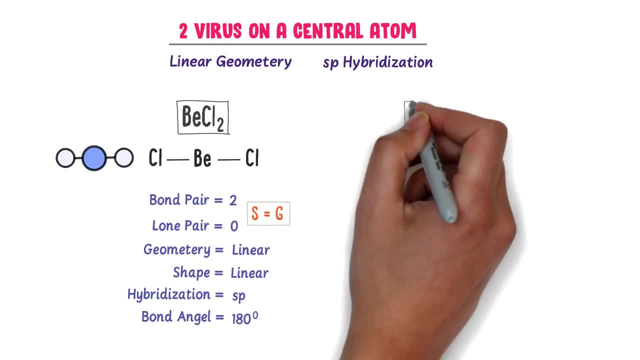 degree. Secondly, consider carbon dioxide. The Lewis structure of carbon dioxide is like this. Remember that single bond contains one pair of electrons, while double bond contains two pair of electrons. There are total two bonds present in a carbon dioxide molecule, so there are four bond. 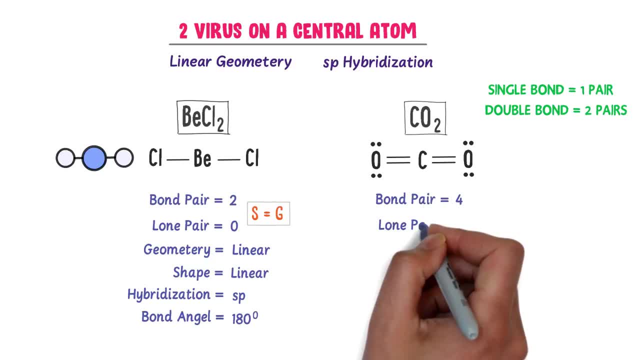 pair of electrons are present in it. There are zero long pair of electrons present on a central atom. The shape of a carbon dioxide molecule is the same as its geometry. Here let me clear one biggest confusion of students. They say that in carbon dioxide molecule there are four long 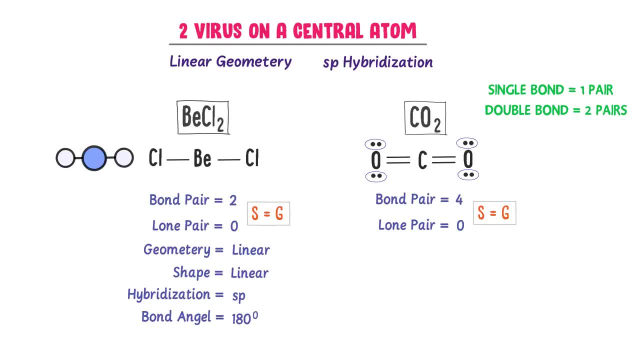 pairs. but it is incorrect. According to whisper theory, long pair of electrons are only considered on central atom like carbon. The long pair of oxygen atoms are not considered. Thus there is no long pair of electrons present in it. Also, the shape of carbon dioxide is the same as its. 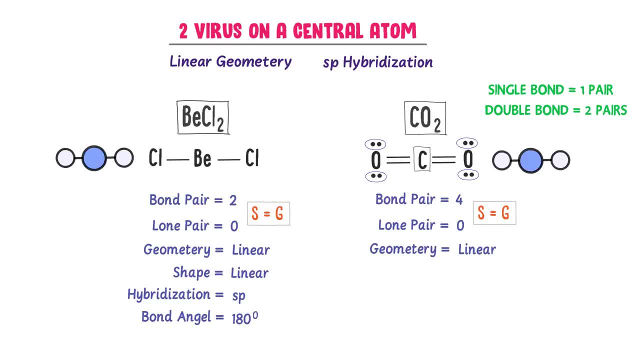 geometry. The geometry of carbon dioxide is linear, so its shape is also linear. It contains SP hybridization. The bond angle of carbon dioxide is 180 degree. Therefore, note it down: the bond pair of electrons, long pair of electrons, geometry, shape, hybridization. 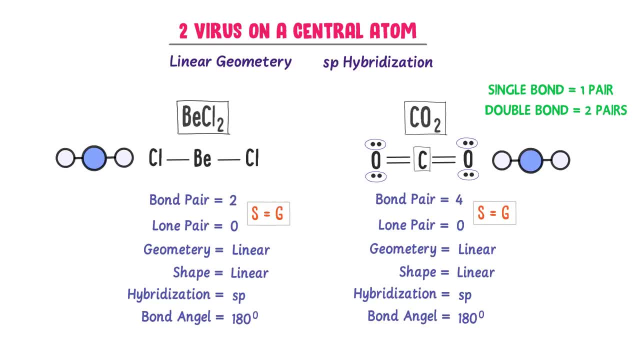 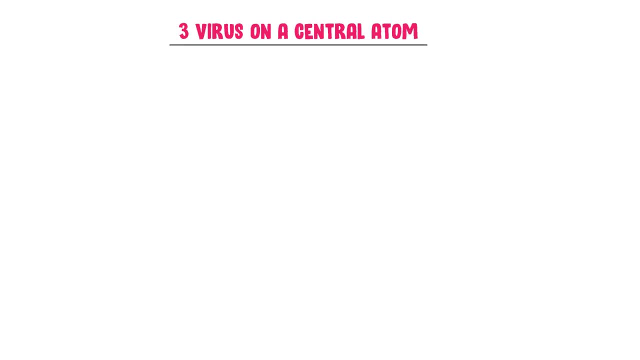 and bond angle of these two molecules. Secondly, consider molecules where there are three atoms or three wires present on a central atom. The geometry of these molecules are trigonal planets. The geometry of these molecules are trigonal planets. The geometry of these molecules. 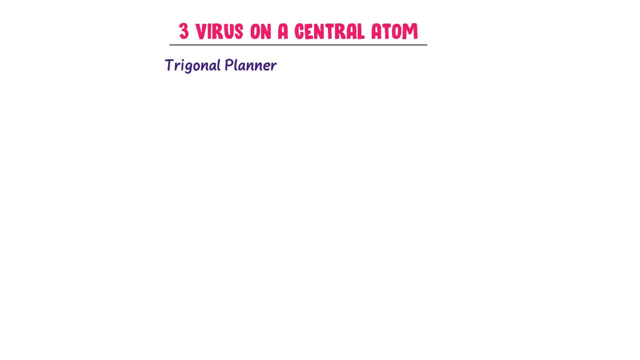 is linear and it never changes. These molecules contain SP2 hybridization. For example, consider molecules like BF3.. The Lewis structure of BF3 is like this: There are three single bonds present in it, So the bond pair of electrons in it is three, So there are three bond pair of electrons. 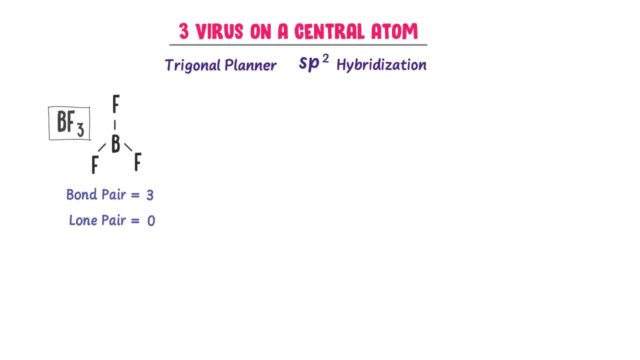 present in it. There is zero long pair of electrons present in BF3.. Thus the shape and geometry of carbon dioxide is the same as its geometry. The geometry of BF3 is the same. The geometry of this molecule is trigonal planar, for example. 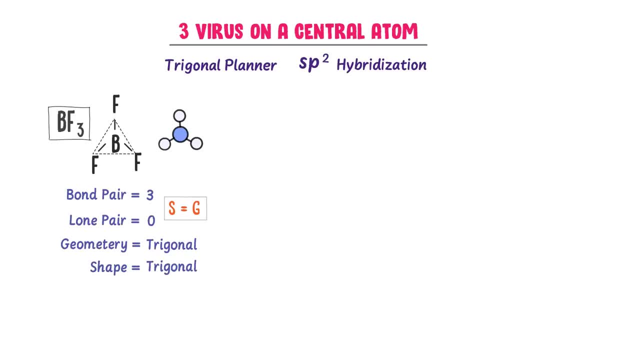 like triangle. The shape of BF3 is also trigonal, planar. The hybridization in BF3 is SP2 hybridization and the bond angle is 120 degree. Now what about sulfur dioxide, SO2?? Well, this is the Lewis structure of sulfur dioxide. There are three things. 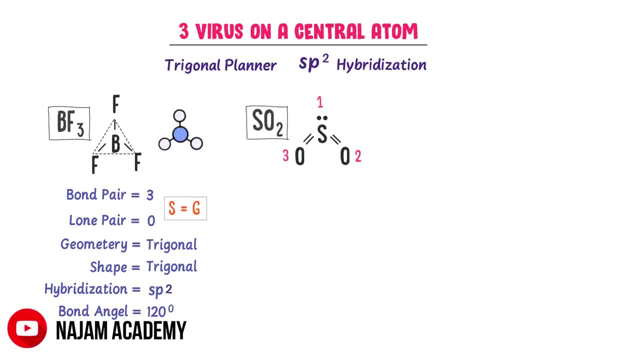 or three viruses present on the central atom. In sulfur dioxide there are two single bonds present, So the bond pair of electrons in it is two. This is the long pair present on a central atom, So there is one long pair present in sulfur dioxide. According to whisper theory, the shape 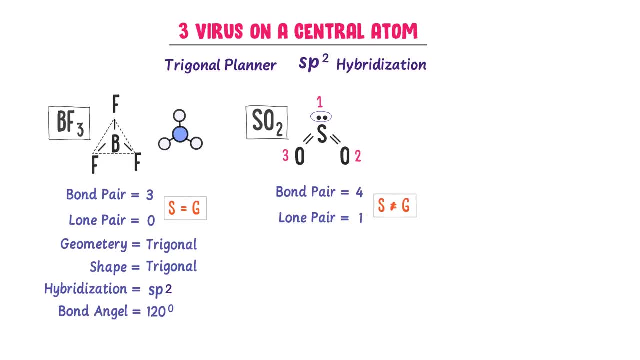 of a sulfur dioxide molecule would be different from geometry of sulfur dioxide. There are three biologies present, and they were AO1,слиph group, which is sea System, and SEA and Webbian Belgium, which is Edebium League, and there are three other biologies present. 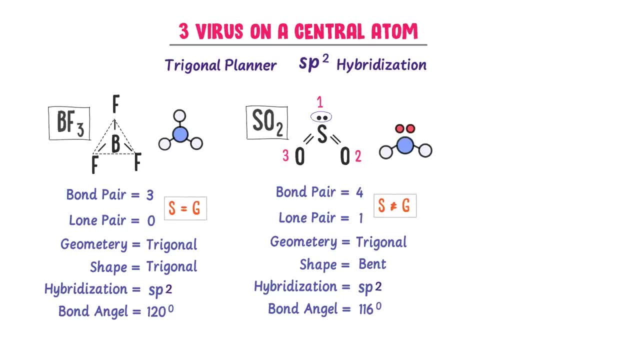 Here there are three biologies present in the volume AB2 and the overscope. Some of them are located at haggon. between the motions the bond angle is 116 degree. Can you guess the reason why the bond angle decreases from 120? 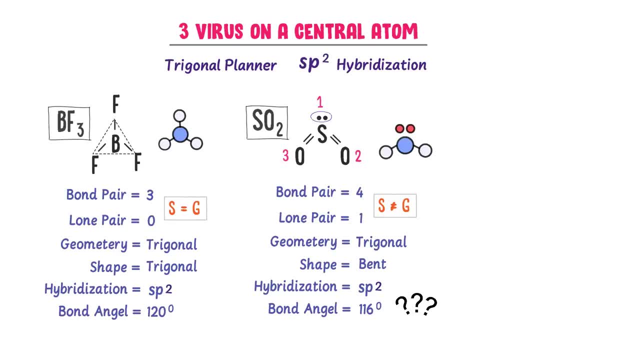 degree to 116 degree. Well, here comes the application of whisper theory. We have learnt in the main points of whisper theory that there is maximum repulsion between lone pair and bond pair of electrons, then bond pair and bond pair of electrons. So this lone pair of electrons on 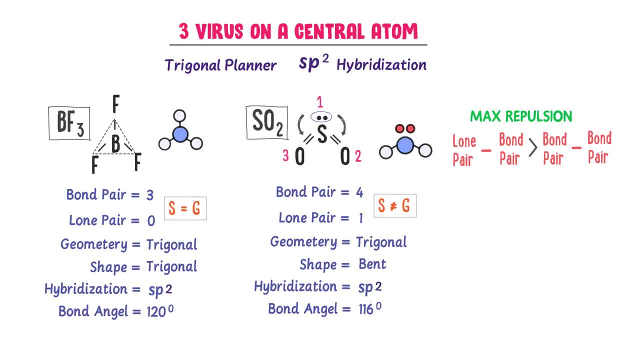 central atom would push the bond pair, thereby decreasing the bond angle from 120 degree to 116 degree. Note it down that bond angle is decided by both the bond pairs and lone pair of electrons. Thus, the bond angle is 116 degree in sulfur dioxide due to lone pair on a central atom. 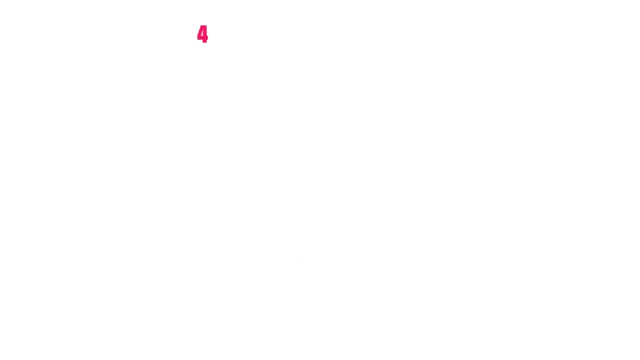 Thirdly, consider molecules where there are four atoms or four virus present on a central atom. The geometry of all these molecules would be tetrahedral and they would contain sp3 hybridization. Also, we know that the geometry of these molecules remain the same and never changes. For example, consider methane CH4.. The Lewis 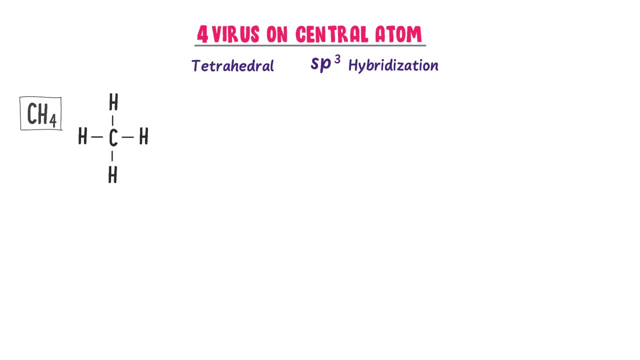 structure of CH4 is like this: There are four single bonds present in it. So there are four pairs present in it. There is no lone pair present in it. So the ship of CH4 is the same as its geometry. The geometry of CH4 is tetrahedral and its ship is also tetrahedral. It contains sp3. 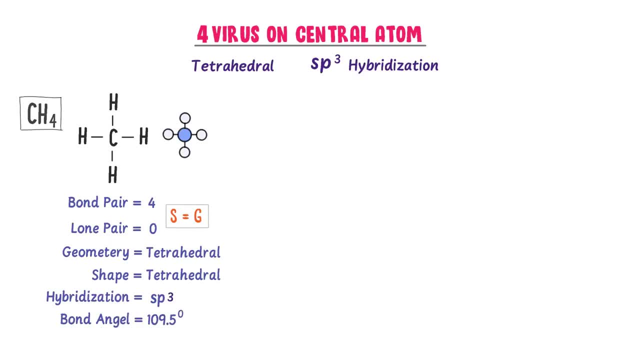 hybridization, and the bond angle is 109.5 degree. Secondly, consider ammonia NH3.. The Lewis structure of ammonia is like this: We can see that the bond angle is 109.5 degree. So the bond angle is 109.5. 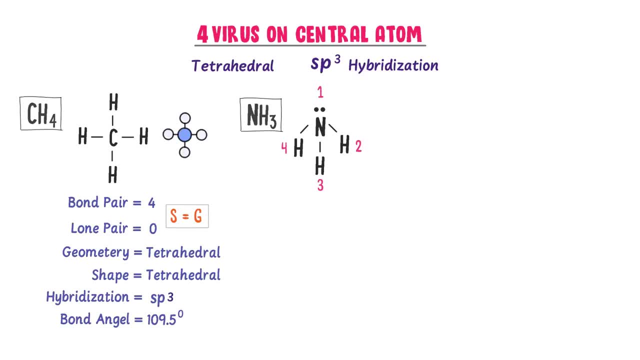 degree. There are four viruses present on a central atom. Nitrogen forms three single bonds with hydrogen, So there are three bond pairs present in it. There is only one lone pair of electrons present. So the ship of NH3 is not the same as its geometry. We know that the geometry 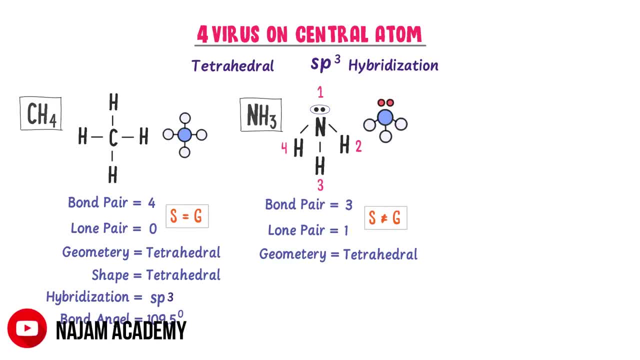 of ammonia. NH3 is tetrahedral. What about the ship of NH3?? Well, hide the lone pair of nitrogen. We can see that the ship of NH3 is pyramidal. There is sp3 hybridization in it. What about the? 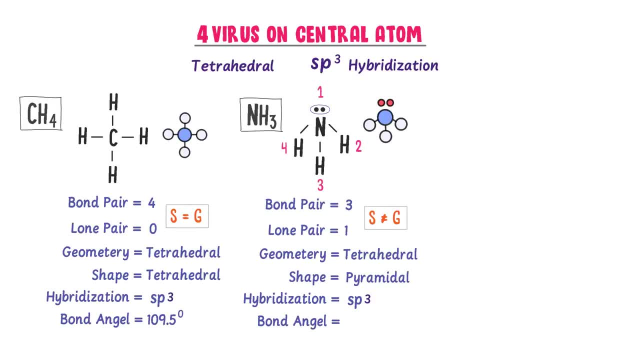 bond angle. Well, the bond angle of NH3 is 107 degree. The angle of CH3 is 109.5 degree, But the lone pair of nitrogen decreases the bond angle from 109.5 degree to 107 degree. Thirdly, consider: